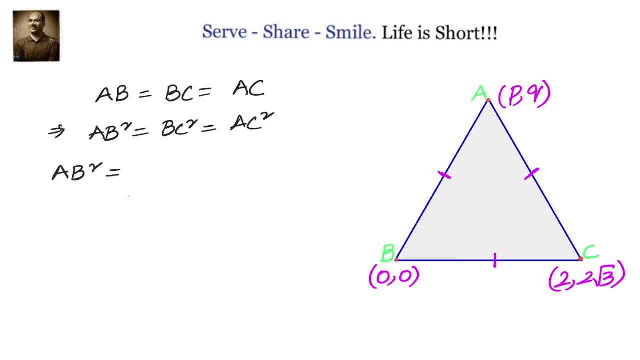 Now let us see what is AB square. AB square is P minus 0 whole square plus Q minus 0 whole square, which is equals to P square plus Q square. that is coming from distance between point A and point B. Now let us see what is AB square. AB square is P minus. 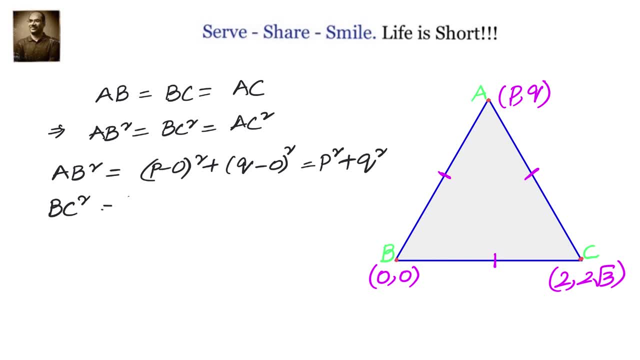 0 whole square plus Q square. that is coming from distance between two points formula. Similarly, what is BC square? BC square is 0 minus 2 whole square plus 0 minus 2 root 3 whole square, which is equals to 2 square plus 2 root 3 whole square. 2 square is 4 and 2 root 3 whole square is 12.. So 16 we get. Let us do AC square now. 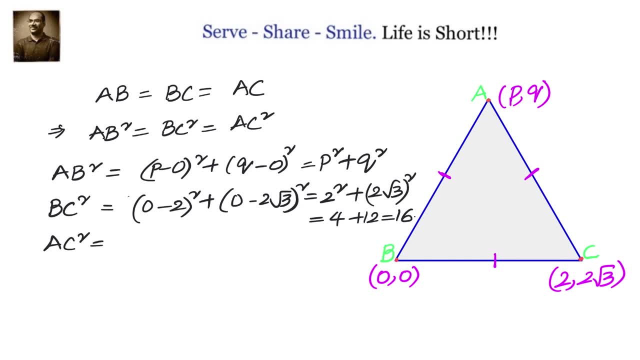 AC square is P minus 2 whole square plus Q minus 2 root 3 whole square. Now let us take and equate them. First, we will equate AB square to BC square. We will get P square plus Q square equals to 16.. 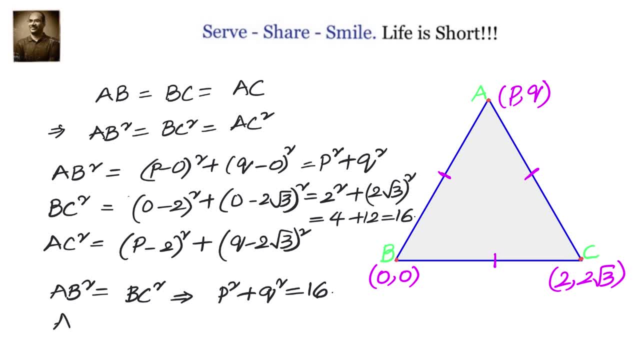 we need another relationship between p and q so that we can solve for the values of p and q. a b square equals to a c square. we will take, we will write down: p square plus q square equals to p minus 2 whole square, that is, a minus b whole square. formula identity. so we can write: 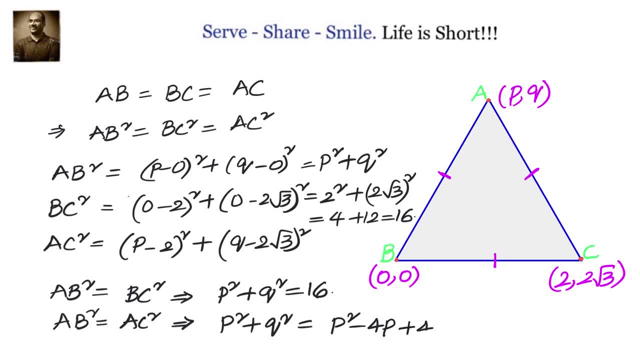 down p square minus 4 p plus 4 plus q square minus 4 root 3 q plus 2 root 3, whole square, that is 12. simplify that. we can cancel p square and q square on left hand side and right hand side. we will get a linear equation in p and q that will be 4 p plus 4 root 3 q. 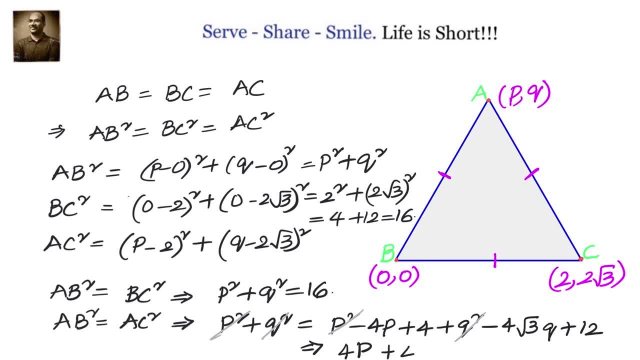 equals to 16, or we can divide by 4 and get the condition as: p plus root 3, q equals to 4. let us document these two conditions because we are going to work on them. one is p square plus q square is 16 and another is p plus root 3. 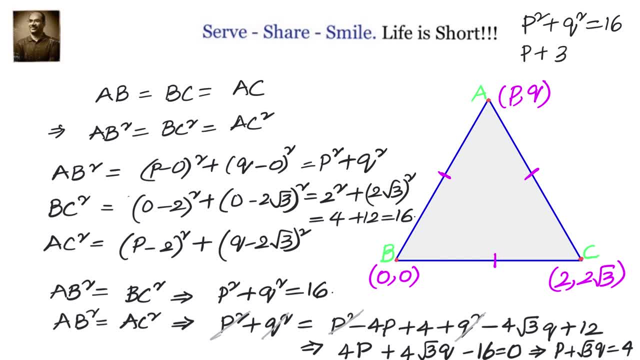 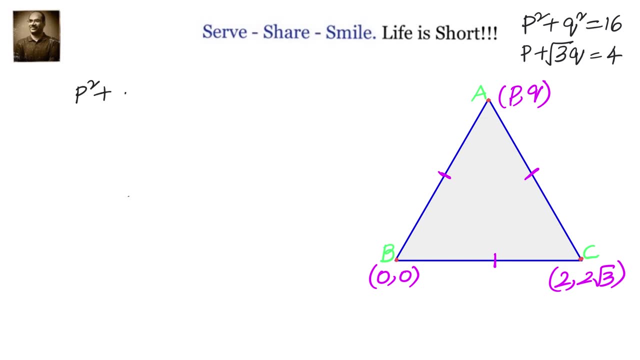 Q equals to 4.. Now we will try to express in terms of P so that we can solve for P. So we will write down: P square plus Q square is 16.. So we can write down. The second equation we have is: P plus root 3 equals to root 3 into Q equals to 4, which we can write it. 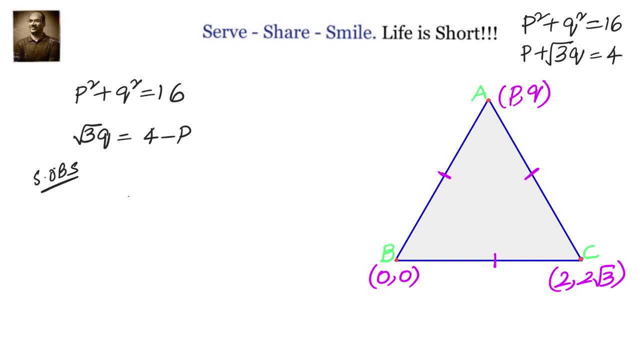 as root 3 into Q is 4 minus P. Squaring on both sides we will have 3. Q square equals to P square minus 8, P plus 16.. Now let us express Q square in terms of P square. So in the next step we will write down: 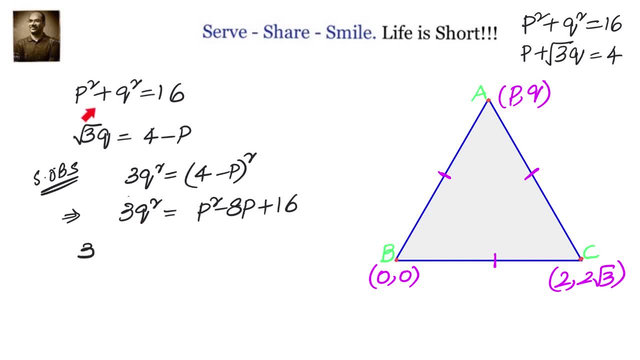 3 into 16 minus P square equals to P square minus 8 P plus 16.. Now we got a quadratic equation in P. Simplify that and let us find out the P values. So we have 48 minus 3 P square equals to P square minus 8 P plus 16.. We are bringing everything from left-hand. 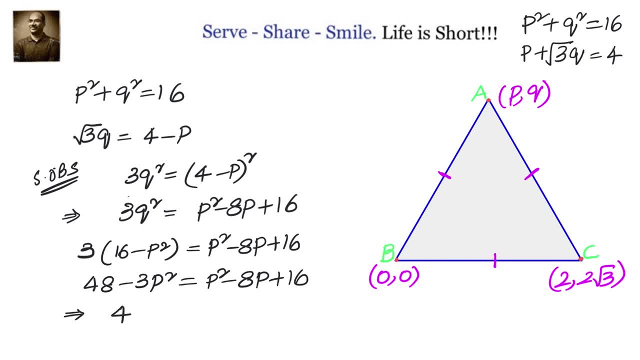 side to right-hand side, We will have 4 P square minus 8. P minus 32 equals to 0.. We can divide by 4 to split the middle terms: P square minus 2. P minus 8 equals to 0, which can be factorized as P minus 4.